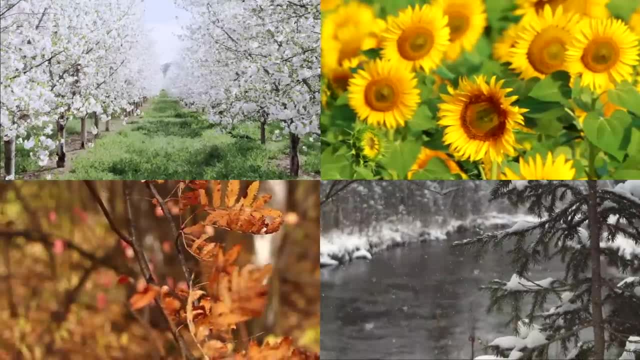 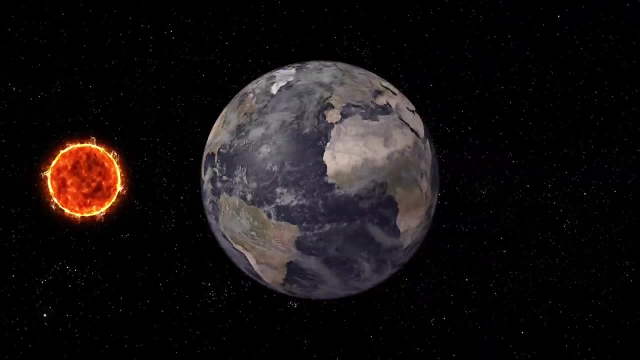 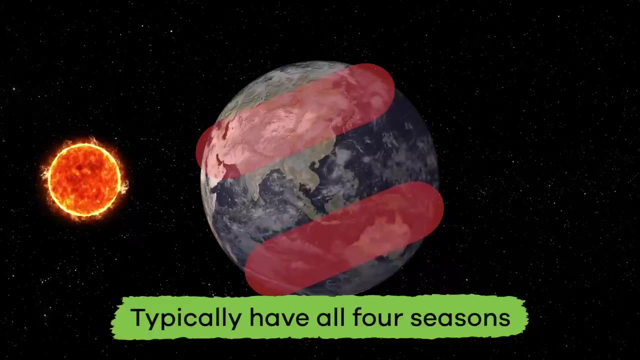 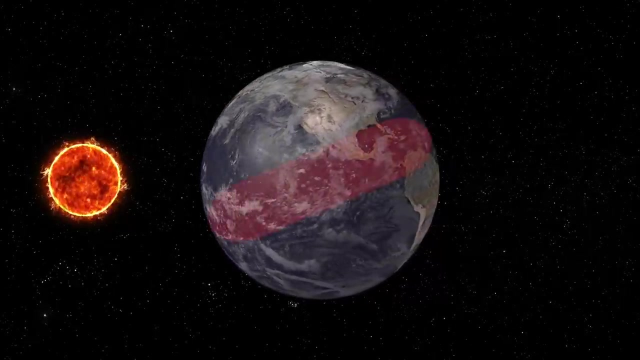 you live, There are four seasons: spring, summer, fall and winter. The parts of our planet that are located halfway between the North and South Poles typically have all four seasons, like a lot of areas in the United States, But this is not true of everywhere In places near the equator. 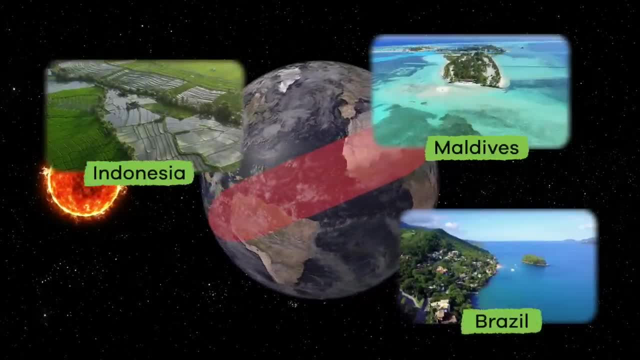 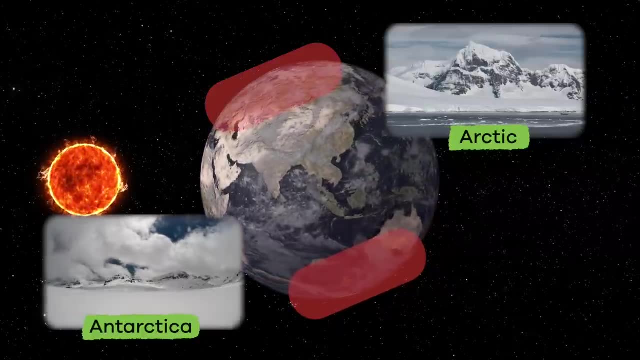 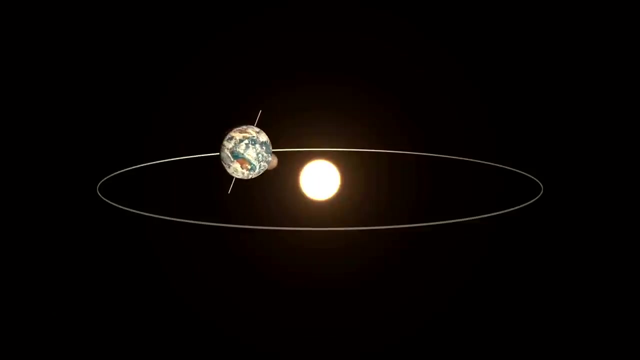 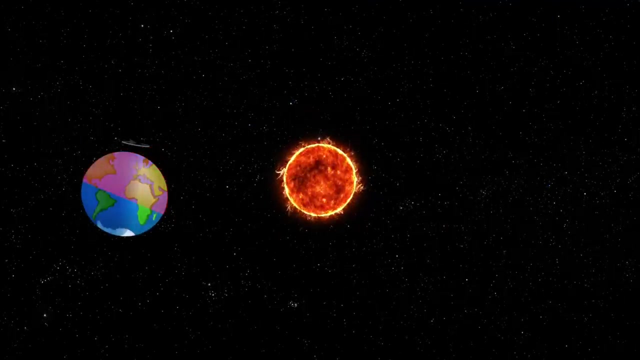 it feels like summer all year round, And in places near the North Pole or the South Pole it always feels like winter. Remember when we mentioned that seasons are related to the earth's rotation. Now we are going to show you how. When the earth rotates around the sun, one half or hemisphere- 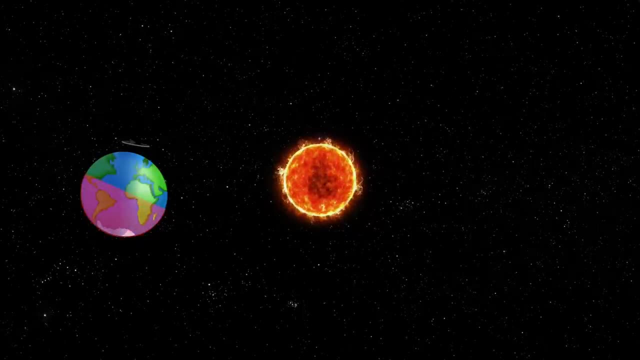 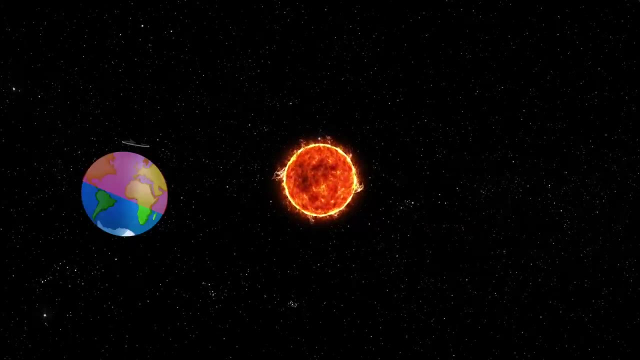 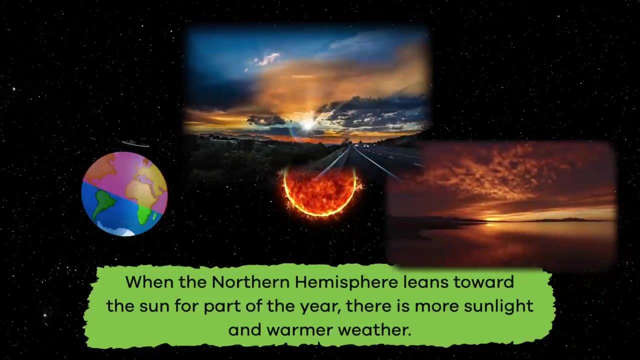 leans toward the sun and the other half leans away. Let's look at the Northern Hemisphere, or top half of the earth, as an example. When the Northern Hemisphere leans toward the sun for part of the year, there is more sunlight and warmer weather. 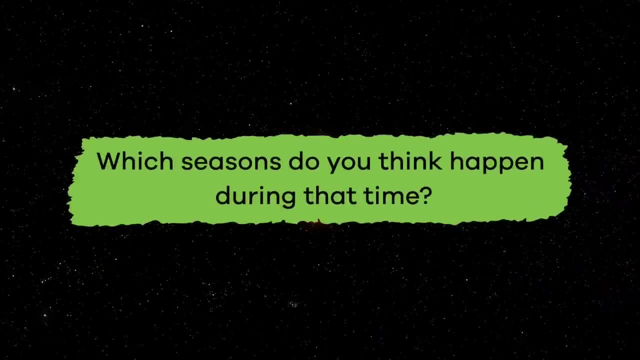 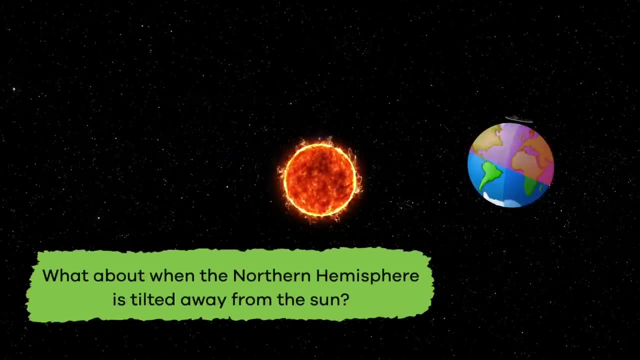 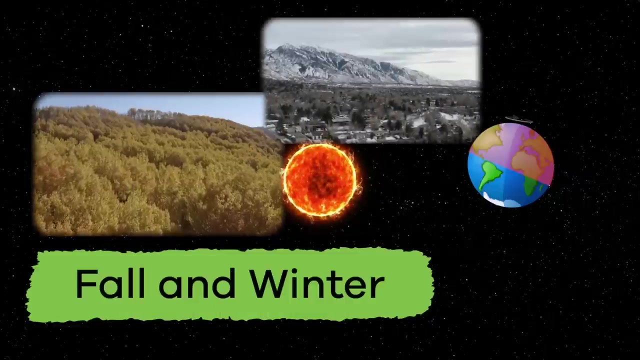 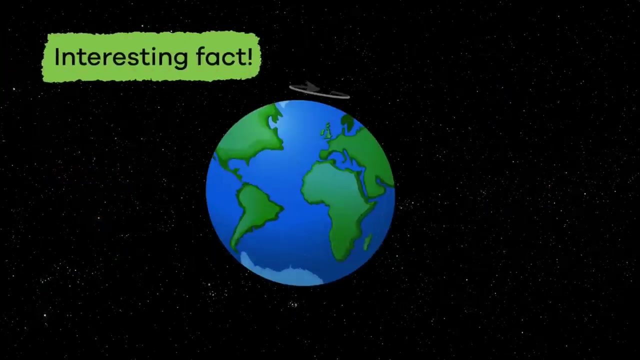 Which seasons do you think happen during that time? That is right, The seasons are spring and summer. And what about when the Northern Hemisphere is tilted away from the sun, With less sunlight and cooler weather? it is definitely time for fall and winter. Here is an interesting fact: When it is summer, 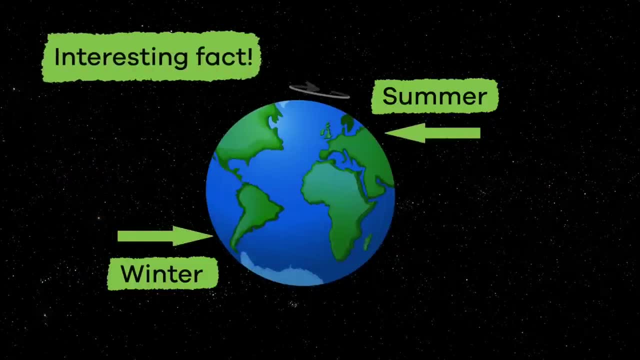 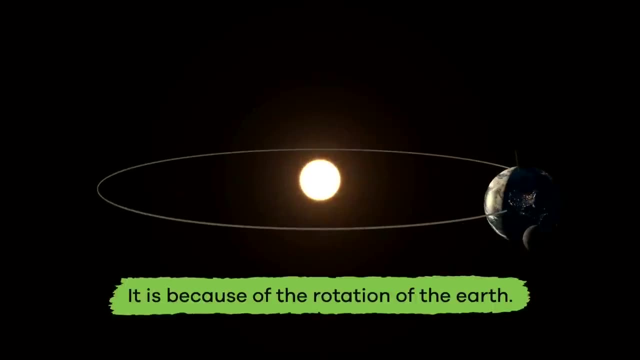 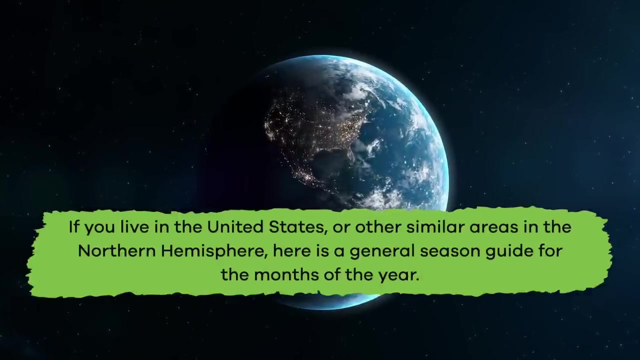 in the Northern Hemisphere. it is winter in the Southern Hemisphere, and vice versa. And why is that? It is because of the rotation of the earth. If you live in the United States or other similar areas in the Northern Hemisphere, here is a 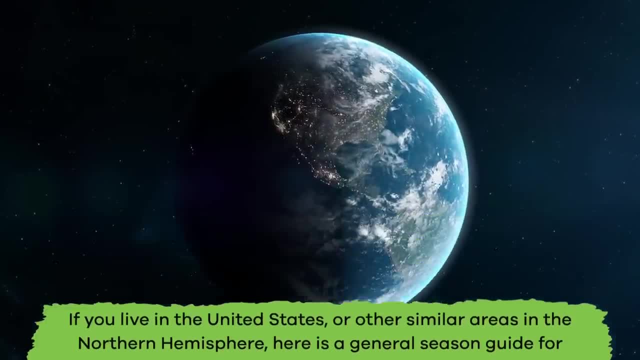 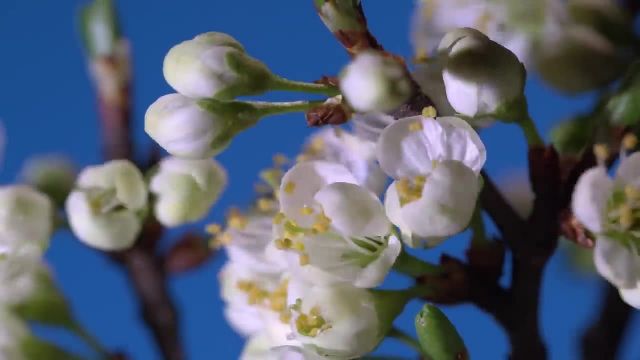 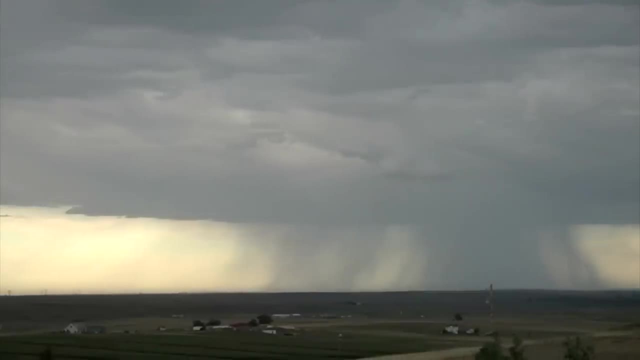 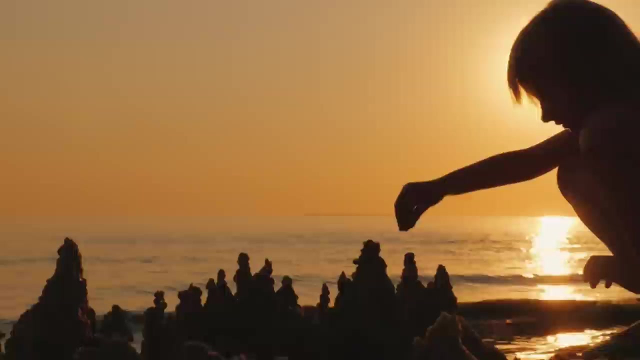 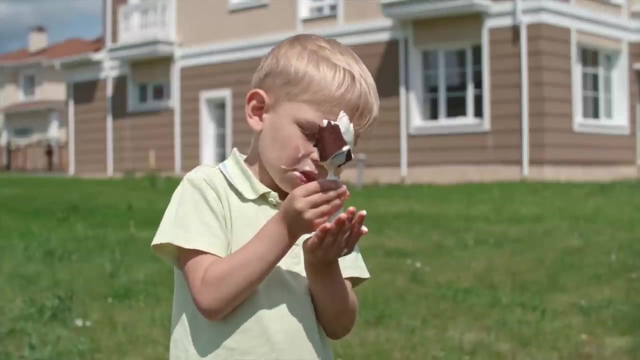 general season guide for the months of the year. If you live in the United States or other similar areas in the Northern Hemisphere, here is a general season guide for the months of the year. Let's take are the¬¬¬¬¬¬¬¬¬¬¬¬¬¬¬¬¬¬¬¬¬¬¬¬¬¬¬¬¬¬¬¬¬¬¬¬¬¬¬¬¬¬¬¬¬¬¬¬¬¬¬¬¬¬¬¬¬¬¬¬¬¬¬¬¬¬¬¬¬¬¬¬¬¬¬¬¬¬¬¬¬¬¬¬¬¬¬¬¬¬¬¬¬¬¬¬¬¬¬¬¬¬¬¬¬¬¬¬. 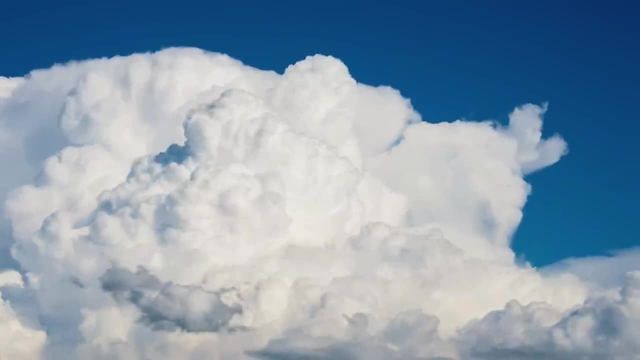 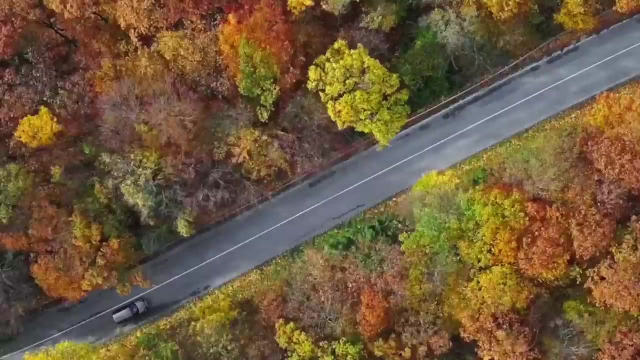 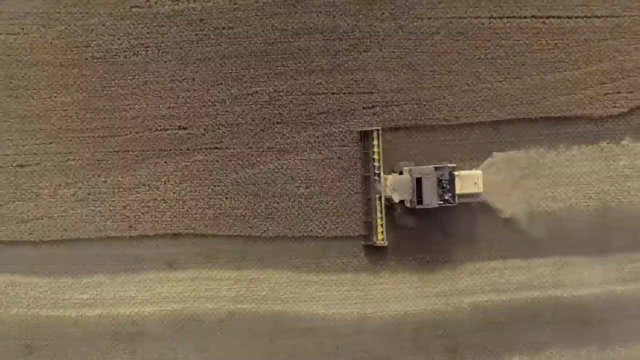 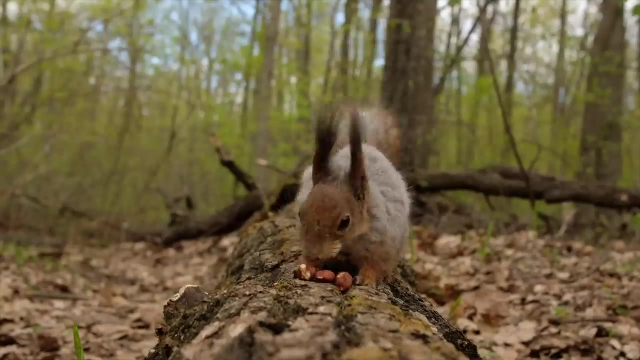 grow taller and bigger, and you might notice more thunderstorms too. Fall – September, October and November. Fall is the beginning of the colder months, when temperatures start to fall and crops are ready to be harvested. This is also the time when animals start gathering food for the winter months and when the leaves 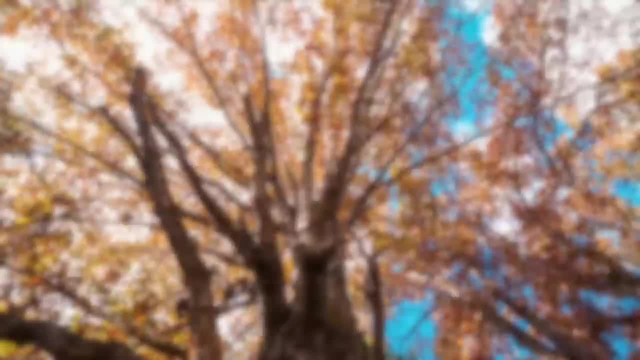 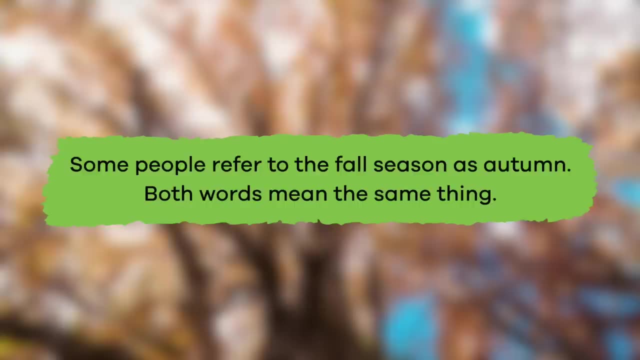 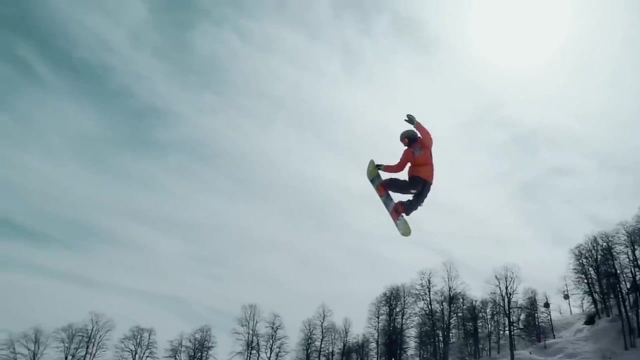 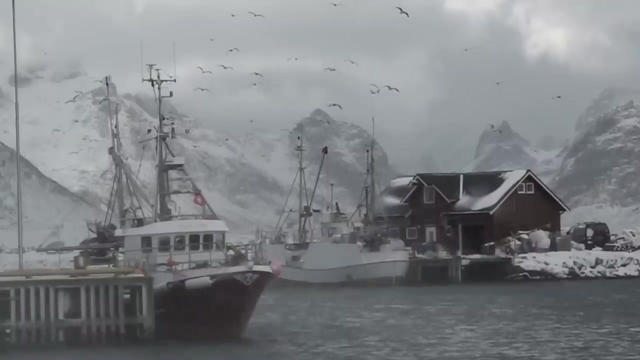 on trees change colors. Some people refer to the fall season as autumn. Both words mean the same thing Winter –, December, January and February. Last but not least is winter. This is a time when most plant life is dead or does not bloom. 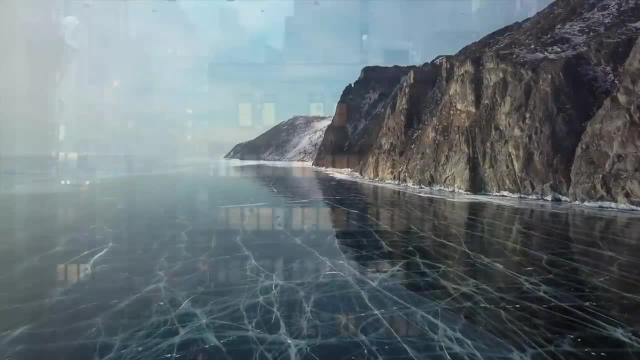 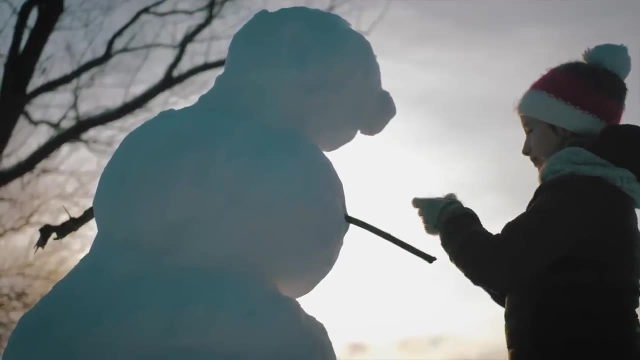 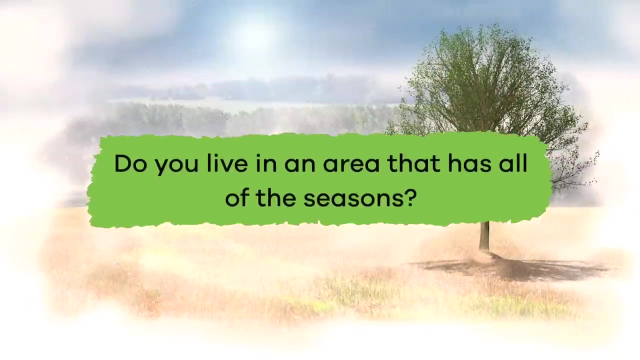 Snow, ice and freezing rain can all happen during the winter, But it is also the time of the year when you can do fun outdoor activities like skiing, ice skating and sledding. Do you live in an area that has all of the seasons? 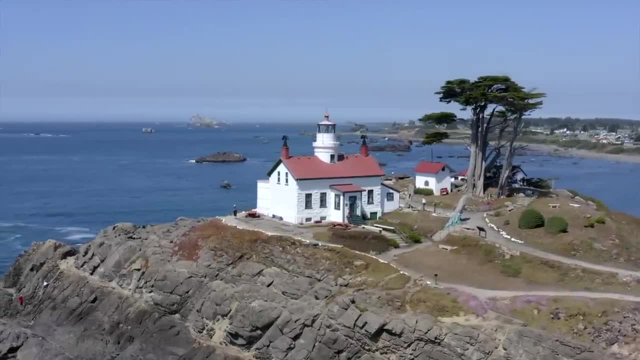 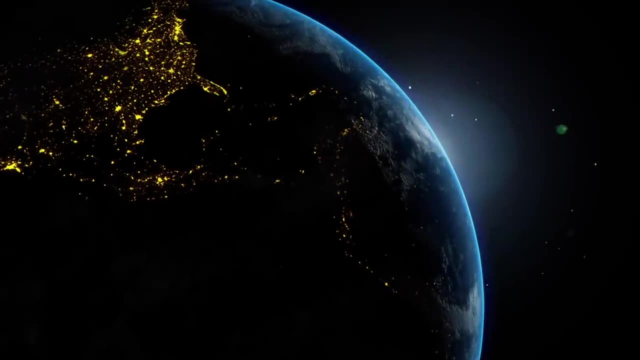 Even if you live somewhere warmer or colder, you might still notice slight changes during the year, even if they are not super dramatic. Who would have thought that our location on the Earth would be so dramatic? Who would have thought that our location on the Earth would be so dramatic? 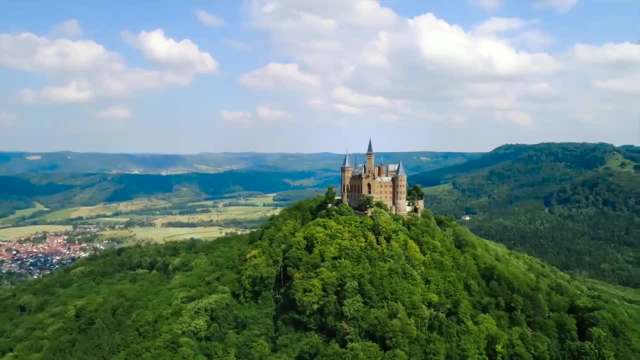 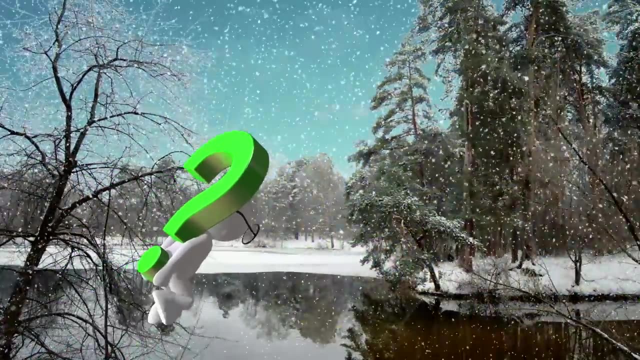 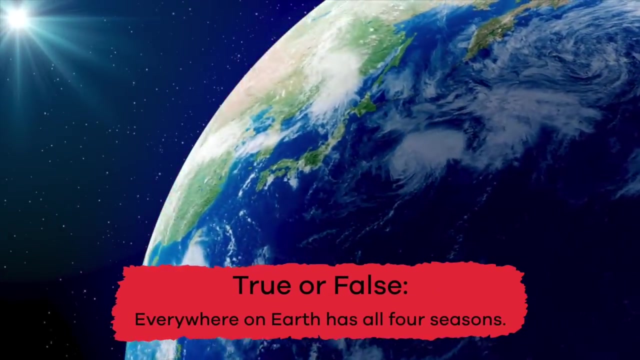 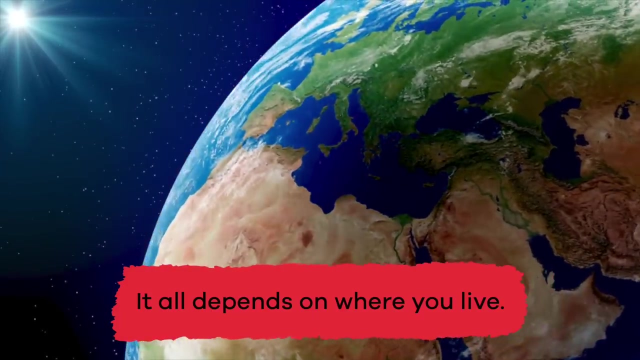 Who would have thought that our location on the Earth would be so dramatic. Let's review TRUE or FALSE. Everywhere on Earth has all four seasons. FALSE. It all depends on where you live. FILL IN THE BLANK SEASONS. 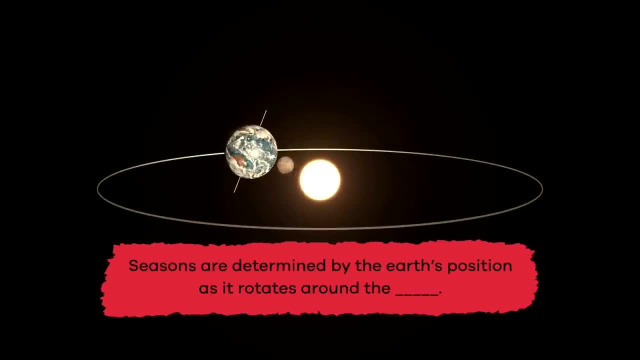 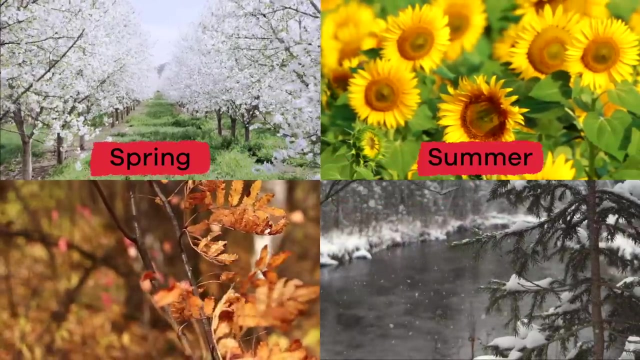 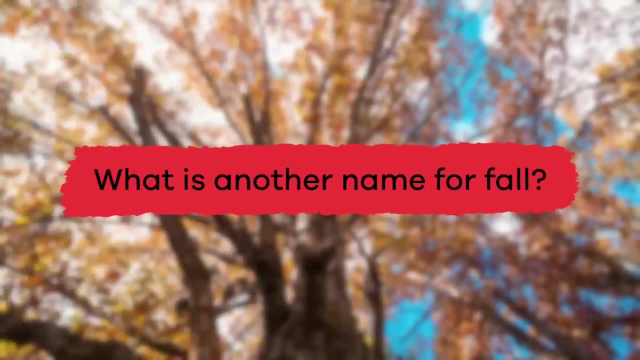 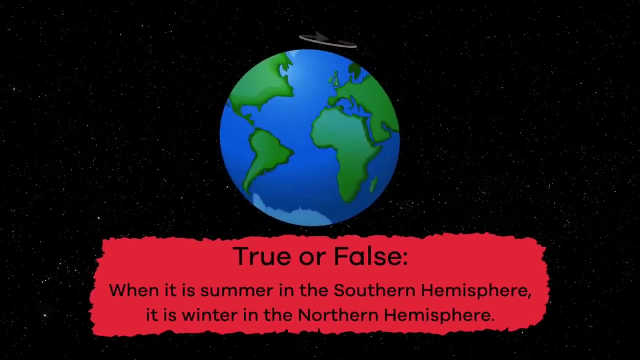 Seasons are determined by the Earth's position as it rotates around the blank, The Sun. Name all four seasons: Spring, Summer, Fall and Winter. What is another name for Fall, Autumn, True or False? When it is summer in the Southern Hemisphere, it is winter in the Northern Hemisphere.